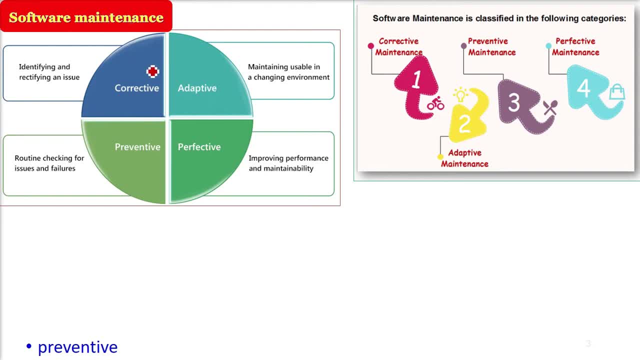 Software maintenance takes various types. This can be done in 4 types: Preventive- I have written first because this is more related to the hardware stuff, But still, if you are being asked, you have to talk about all these in software maintenance as well. Software maintenance, or keeping this software up to date. we need certain maintenance First is corrective, adaptive, perfective and preventive. 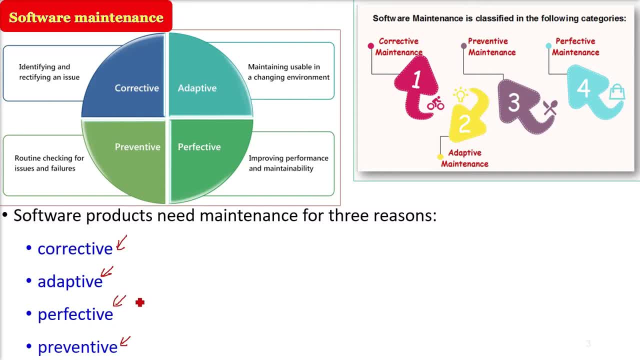 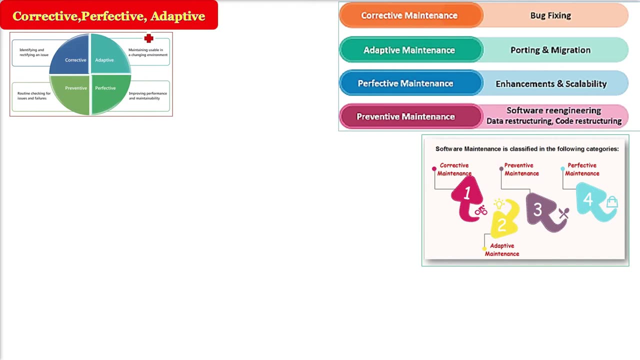 Corrective, adaptive, perfective, preventive. Preventive is the first kind of maintenance, Because this is the fire cannot happen. Corrective is fire happens, then you do certain thing to get away from it. So corrective maintenance, adaptive maintenance, perfective maintenance and preventive maintenance, These are the 4 types of the software maintenance. 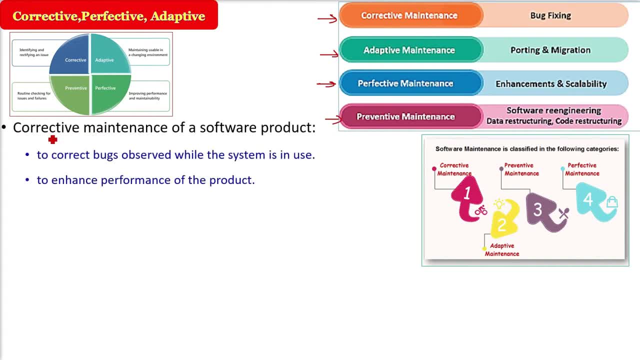 Corrective maintenance is all about bug fixing. So corrective means to correct it. That means something is wrong. If something is wrong, you need to correct it. If you deliver the software to the user now, user start using it. Now user observed that, oh, there are certain problems here, So he will come back to you. He will say, oh, I am facing problem here. Now you will fix the bugs. 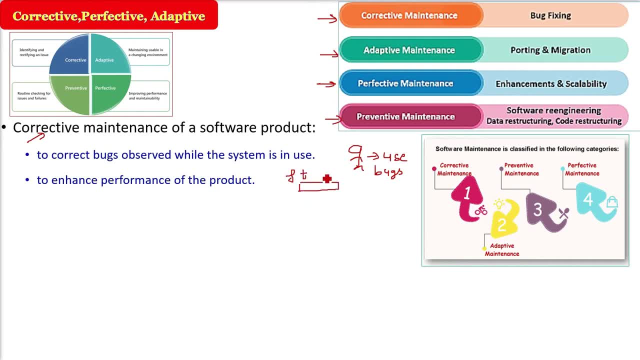 Then, for example, file transfer: you have given Now the speed you wanted. you are not getting it. You will again go back to the developer and you will say, oh, I need enhancement in the performance. So this is a kind of corrective maintenance. 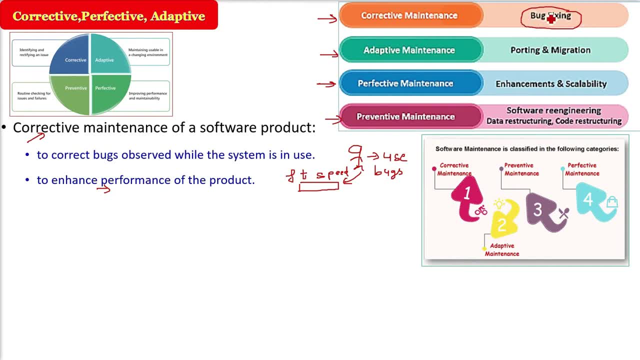 Well, it comes under perfective also, But this corrective maintenance is correction of certain things. What is perfective maintenance? Perfective maintenance is all about enhancements and scalability That is user is using. Now he wants oh. he say, oh, these features are missing. I need these features. Without this, I will not be able to work. 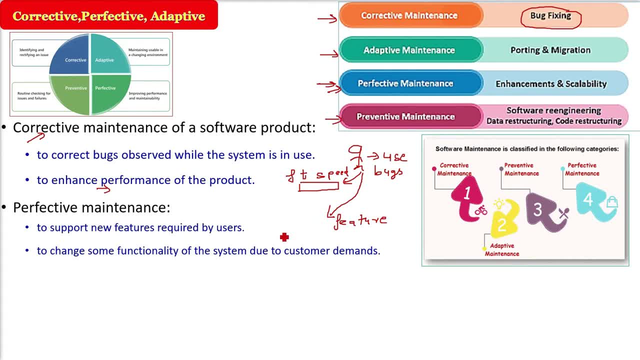 So perfective is the new features, addition required by the user Or certain functionality he is using. he is saying, oh, it should be on the left, not the right, Or I need to change this functionality. So the customer demands the change in the functionality and that when you do that is called as a perfective kind of maintenance. Okay, So it's all about enhancement and scalability in perfective maintenance.